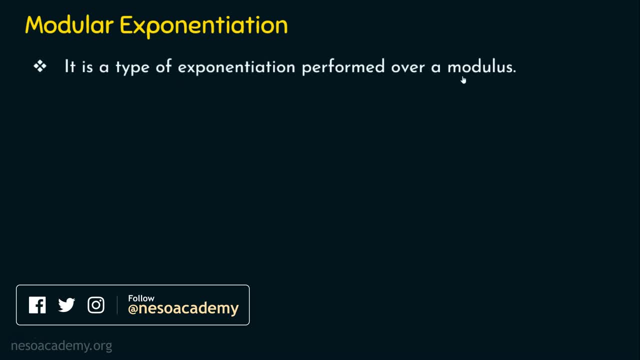 it is a type of exponentiation performed over a modulus. It's not simply x power y we are going to calculate. Rather, we are going to calculate x power y mod m. In other words, we are going to calculate a power b mod m, or this can be represented as a power b. 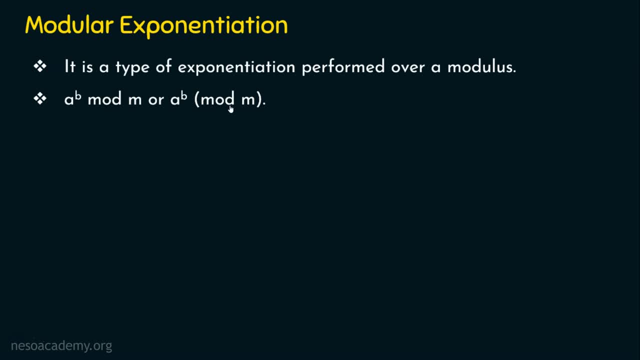 in brackets: mod m. See, please note here why we are using bracket is that it means mod m is not for b, It's for a power, b. Okay, for the whole term, we have mod m, and that's why, in order to 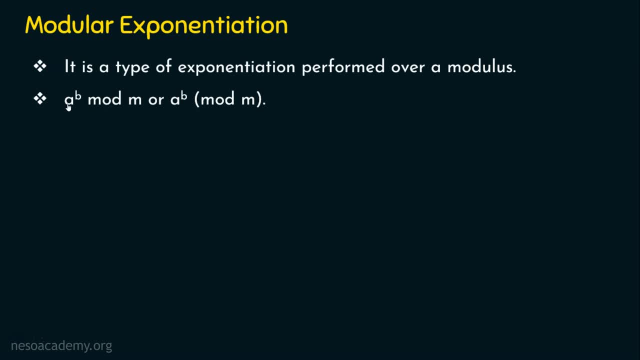 avoid confusion, we use bracket. So whenever it is a power b mod m, it means this mod m is for a power b only, not simply for b. It's for a power b. Let's see some examples. The examples include number one: it's 2 power 33 mod 30.. Let's see: 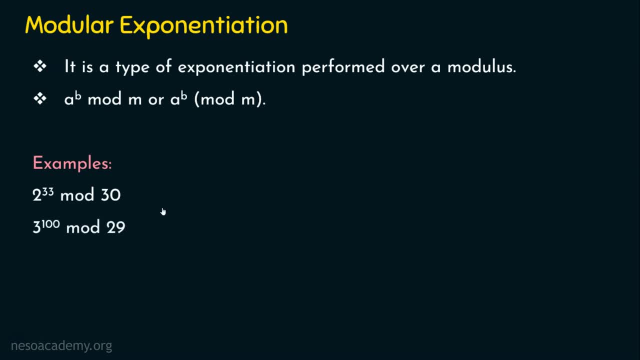 one more example. It is 3 power 100 mod 29.. Let's first start with example number one. The question is: solve 23 part 3 mod 30. So we are going to solve the examples from the base level. 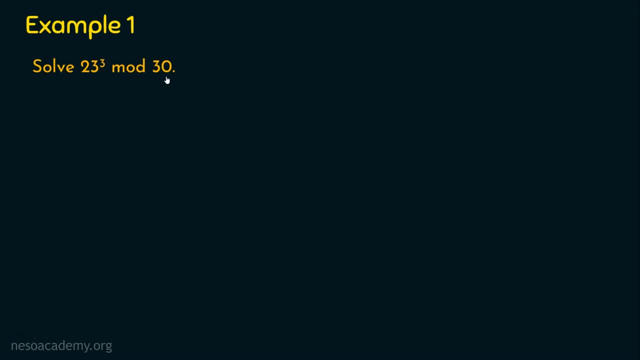 Firstly, we will start with some simple examples. Then we will progress to some complex examples. Firstly, I am starting with 23, part 3, mod 30. It's also easy to do this. You can take a calculator, you can perform 23, part 3 and you will get the result. 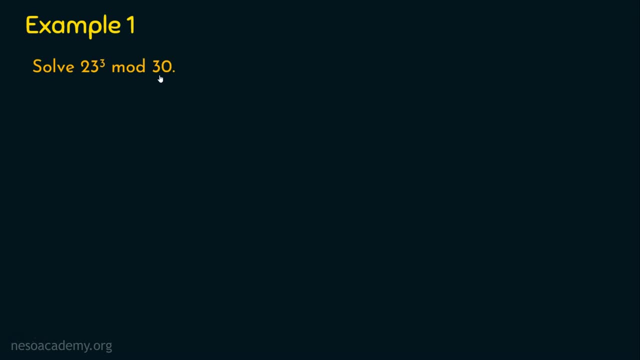 Then divide it by 30 and whatever you get that remainder. It's the answer for this question, right? But I want everyone to try without calculators. That's the main agenda of modular exponentiation. Even big calculations can be easily performed using modular exponentiation. 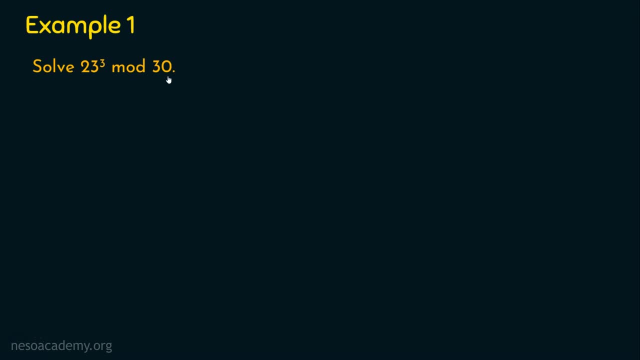 So I strongly recommend you not to use calculators for doing these kind of modular exponentiation problems. Just see how I am doing So we are obviously going to do 23, part 3, mod 30, right, That's what it is given in the question. As mentioned in the previous lecture, there are multiple ways to. 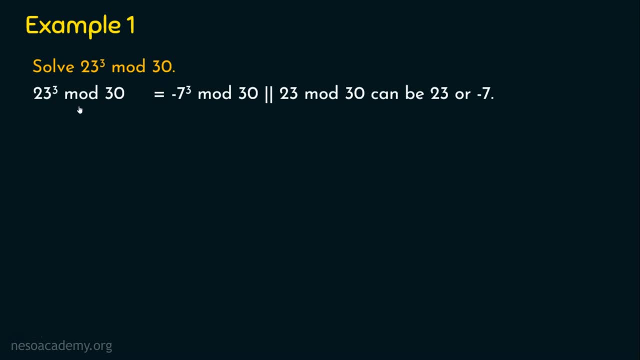 approach a problem, and there are multiple ways to get the solution for that problem, isn't it? You can prefer any approach, but please ensure that the mathematical fundamentals are completely followed. Just see here: 23, part 3, mod 30.. As I already told you, you can start with 23, part 1,. 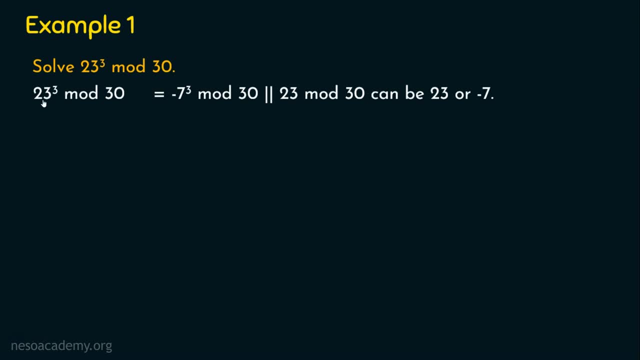 then 23 part 2, then 23 part 3, then 23 part 3.. part 3, or you can simply calculate 23 part 3. whatever you get, that can be divided by 30 and the remainder will be the result, obviously. But see here how I am doing this. This is 23, this is. 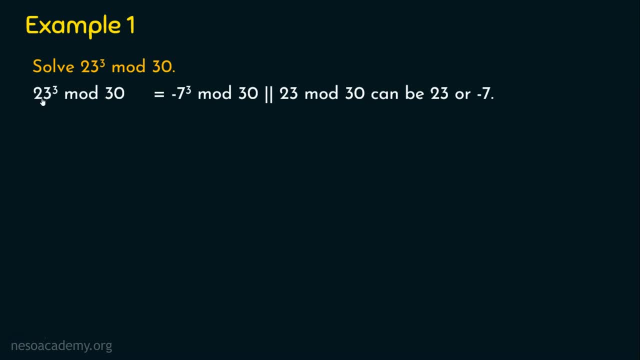 30, right? I can simplify this one with a small number, right? Simply imagine there is no 3 in the power now. It is simply 23 more 30.. 23 more 30: the result will be 23 or minus 7, right? So what? 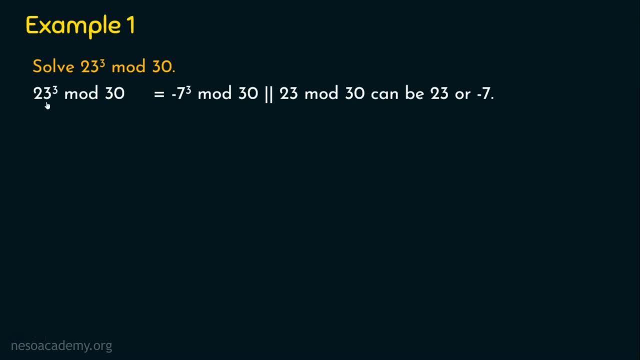 I am doing is I am replacing this 23 by minus 7.. Why? Because 23 more 30 can be 23 or minus 7.. In these two values I can see minus 7 is the smaller value. So I am taking minus 7 power 3. 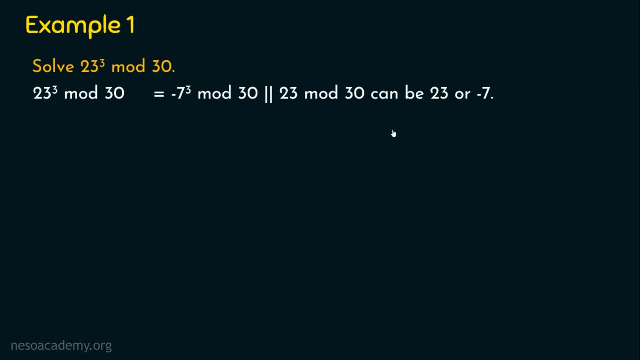 more 30. Now you can easily perform calculation for minus 7 part 3, right? So minus 7 part 3 only. I am preferring. Minus 7 power 3 can be still reduced as minus 7 power 2 into minus 7 power 1. 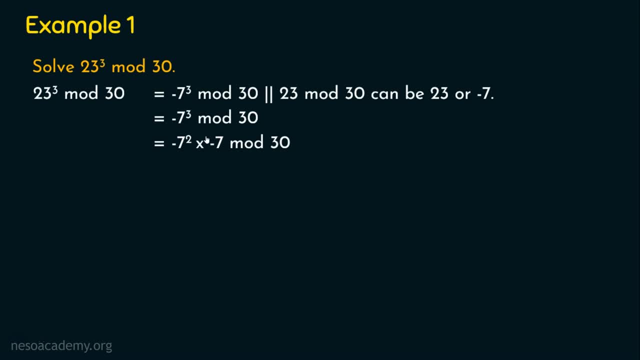 right, We can do this right. When the base is common, you can add the powers right. Here we have the power 3 and the base is common. So I am doing this right, So I am doing this right. So here we have power 2.. Here we have power 1 and the base is common, which is minus 7.. So, minus 7. 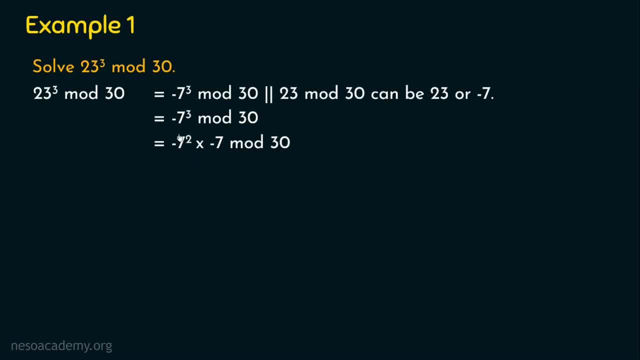 power 2 plus 1, which is minus 7 power 3.. So it is now easy, right? So minus 7 power 2 is what Plus 49, and minus 7 is retained as such, More 30 remains the same. So 49 into minus 7 is minus 133. 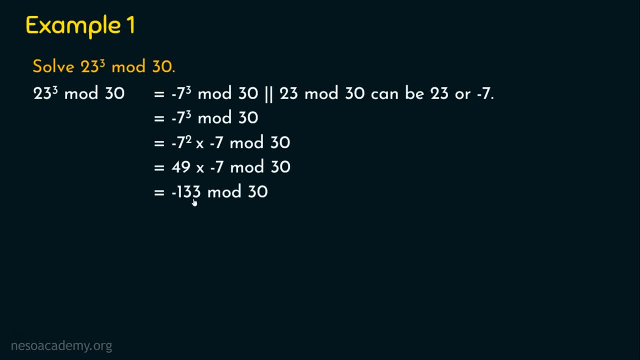 more 30. Now you can easily divide this minus 133 divided by 30. So minus 13 is the answer I already told you always represent the final result as a positive number. So it's so simple to convert this minus number into a positive number. I told. 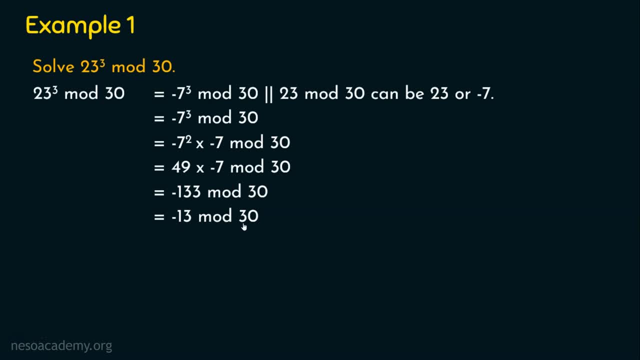 you just add these two values, right? So minus 13 plus 30, it gives plus 17 as the result, right? So I am representing minus 13 with a positive number, 17.. How did I get this So simple? just add this value with this value, So 30 plus minus 13 will give plus 17.. So the answer for this question is: 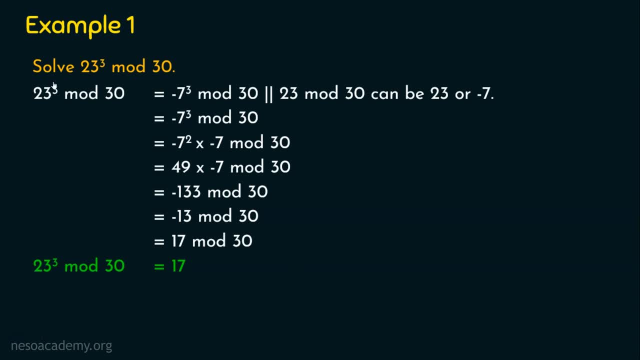 plus 17.. Just see here: I am not going to prefer calculators for calculating 23 power, 3 more 30. Rather, see here: I have simplified this big numbers into small numbers so that I can easily work on the small numbers, and I got the result, Even if 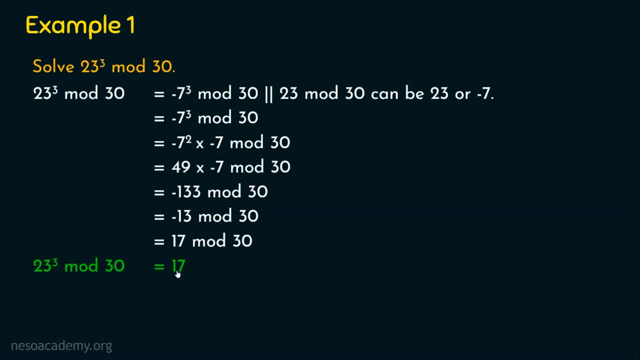 you try with 23, part 3 more 30, you will be getting 17 only as the result. But the difference is we are just working with small numbers. So that's it about example number 1.. Let's now move on to example number 2.. The question is: solve: 31 power, 500 more 30.. 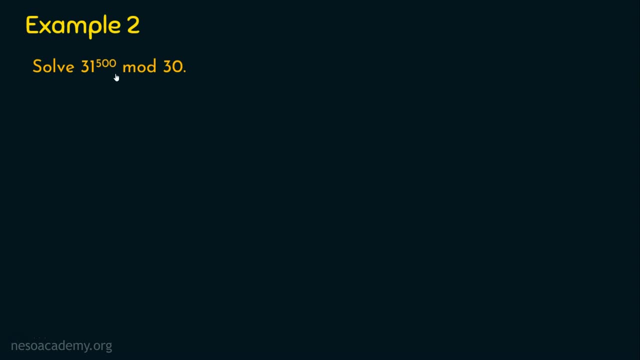 Is it still easy to perform this calculation using a calculator? I will tell you, don't prefer calculator for modular exponentiation, because we can do these jobs simply without calculators. Just see how I am going to do this. So the question is: 31 power 500 more 30, right? So 31 power 500. 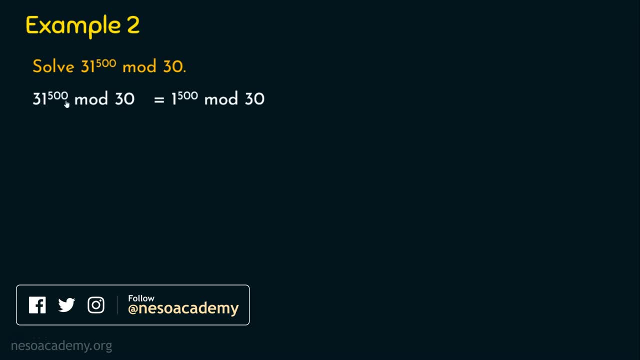 more 30.. No need to do: 31 power 500.. See here how I am doing easily. This is 30, right, more 30, and here we have 31.. So let the power be untouched now, and I am going to replace this 31 with a. 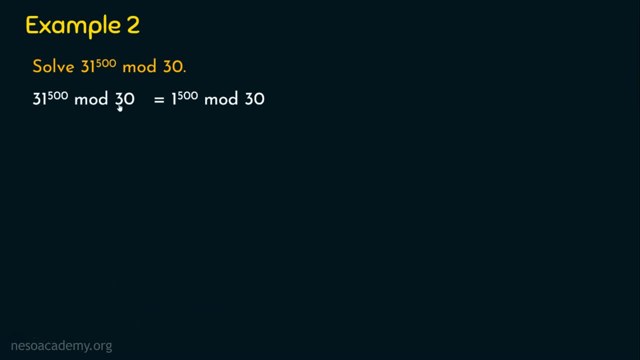 small number. It's like 31 more 30, right? 31 more 30 is what? 31? when it is divided by 30, we get the remainder 1 right. So I am just replacing 31 with 1. now Can you see here? It's so simple you. 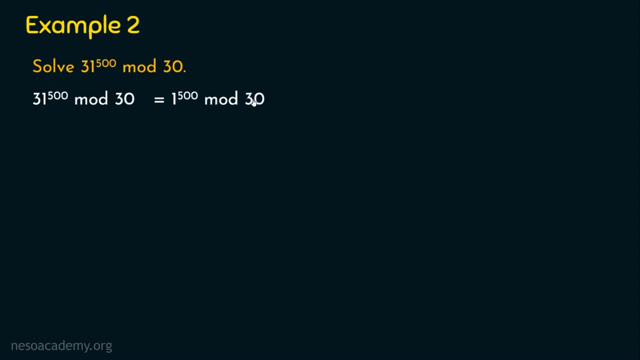 know Now, the question is actually 1 power 500 more 30, right? So 1 power 500 is obviously 1 more 30. So 1 more 30, just divide 1 by 30.. Obviously, the remainder is 1, isn't it? So we have simplified. 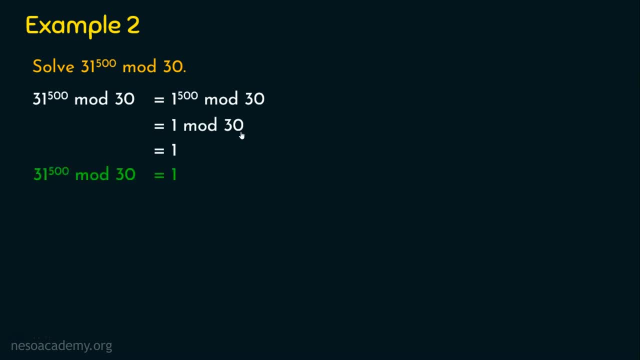 the answer for 31 power 500 more 30 is simply 1.. Isn't it easy. Let's now see another example, Example number 3. In this example, the question is 242 power 329 more 243, and obviously we are. 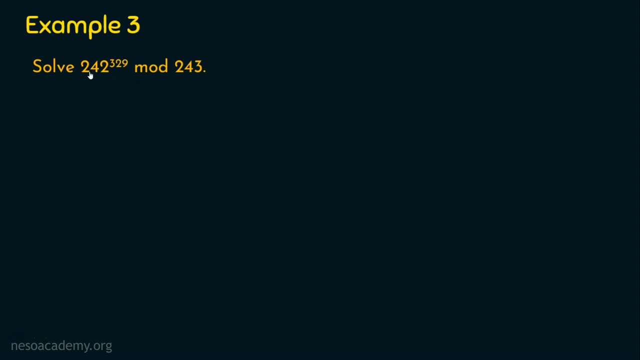 going to do this easily without calculator. See here: it is 242 power 329 more 243.. Obviously, we are not going to seek the assistance of a calculator for simplifying this. Just see here: 242 power 329 more 243. right, See here how easily I am going to do. What is the difference between? 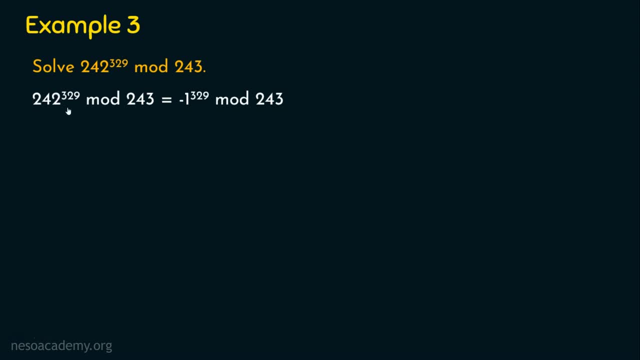 this and this. It's 1 right, This is 1 shortage. So 242 more 243 can be 242 or minus 1.. Which is smaller number? Minus 1 is a smaller number, So I am just taking the smaller number minus 1 here. 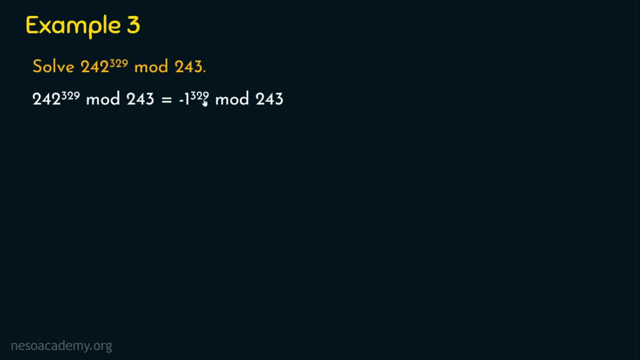 Now the question is: minus 1 power 329.. So minus 1 power 329, it is an odd number, right? So minus 1 number will give minus 1 only, Isn't it? It's so simple. Or we can do like this: Minus 1 power 329. 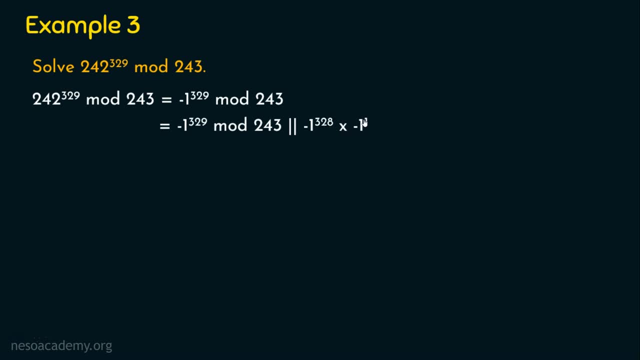 can be written as minus 1 power 328 into minus 1 power 1.. If the base is common, you can simply add the powers, right? So 328 plus 1 is what It's, 329.. So this gives a positive number that is plus. 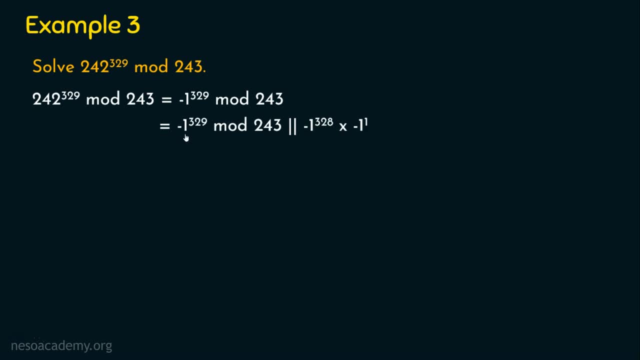 1 and this gives minus 1.. So plus 1 into minus 1 is what Minus 1.. Or you can simply write it as minus 1 power 329 will give you minus 1 only. So the result of minus 1. 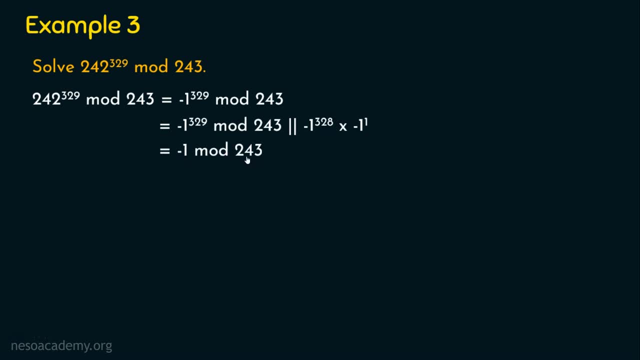 power. 243 is minus 1 only Because it's a smaller number than this number. So you will be getting the same number as the result. I already told you let the final result be represented as a positive number. Just add this minus 1 with 243. We will be getting 242 as the result. So 242 more 243, or. 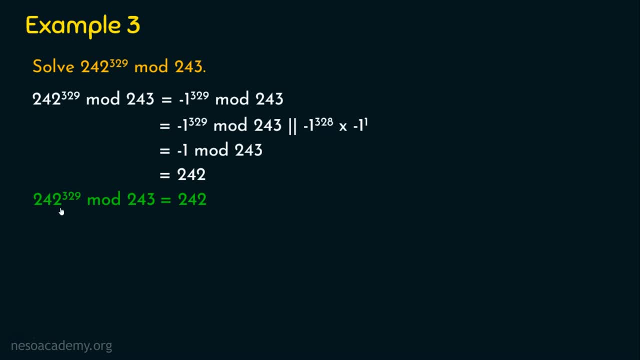 simply 242.. So the answer for 242 power 329 more 243 is 242.. Let's now move on to the last example of the day, Example 4.. The question is solve: 11 power 7 mod 13.. See in the previous case. how did I solve? I can represent. 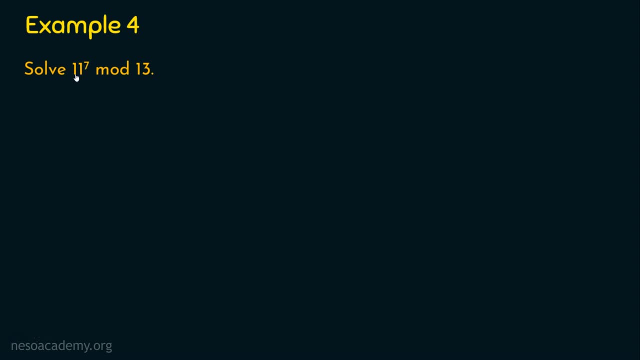 this 11 power 7 as 11 power 7 itself, or I can represent this as minus 2 power 7.. Isn't it So? here I am going to use a different strategy. Just see here how I am doing. 11 power 7 mod 13 can be. 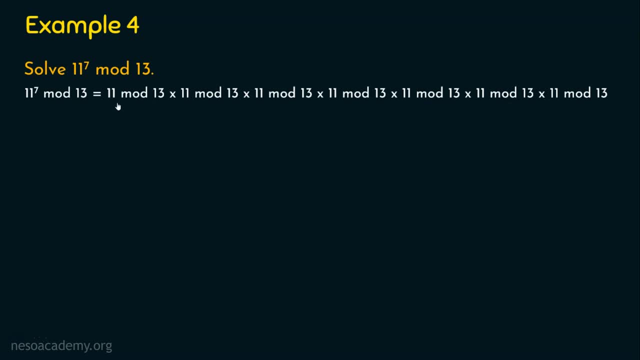 written. as I am multiplying 11 mod 13 7 times, Can you see here? this is 1, 2, 3, 4, 5, 6 and 7.. Now we have 11 power, 7 mod 13.. The result of 11 mod 13 is 11 or minus 2, which is a smaller number, 11 or.